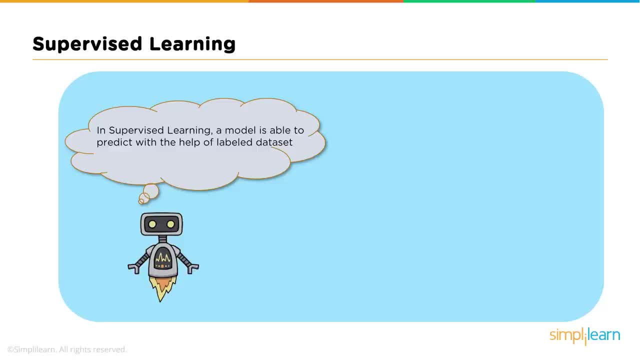 While if I show you an image without telling you what exactly it is, then it's an unlabeled data. Now, let's say we have images which are labeled as spoon or knife. We then feed it to the machine, which analyzes and learns the association of these images. 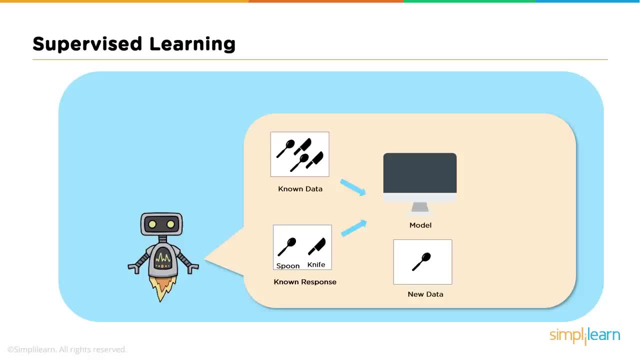 We then feed it to the machine which analyzes and learns the association of these images. We then feed it to the machine which analyzes and learns the association of these images with its labels, based on its features, such as shape, size, sharpness, etc. 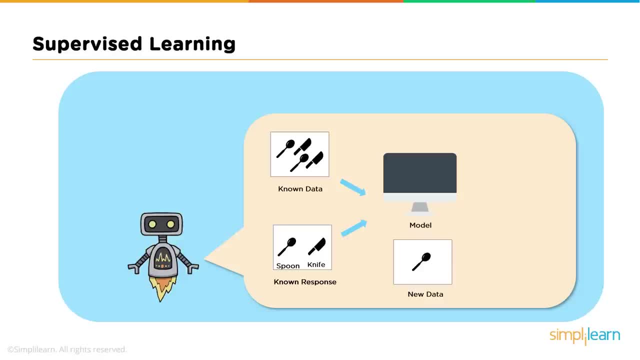 Now, when a new image is fed to the machine without any label, with the help of the past data, the machine is able to predict accurately and tell that it's a spoon Hence in supervised machine learning. the algorithm teaches the model to learn from the labeled example that we provide. 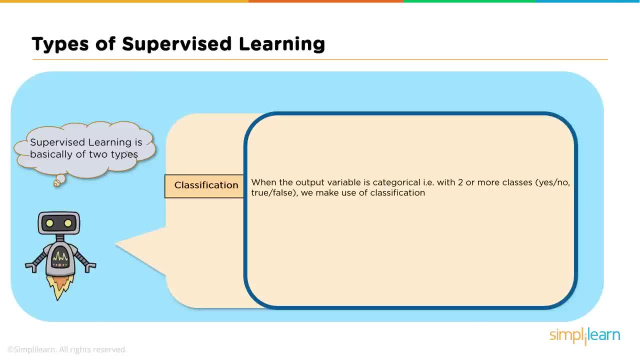 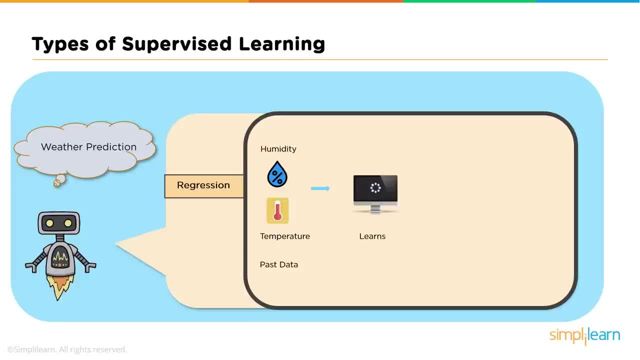 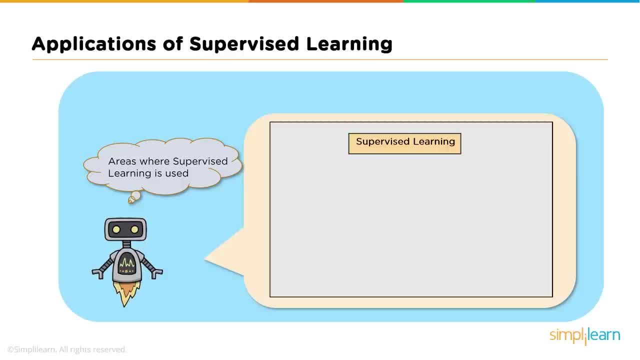 the given temperature. Well, that was about regression. Now let's see some real-life applications where supervised learning is used. So supervised learning is used in risk assessment to assess risk in financial services or an insurance domain to minimize the risk portfolio of the companies. Image classification: Facebook recognizes your friend in a picture from an album. 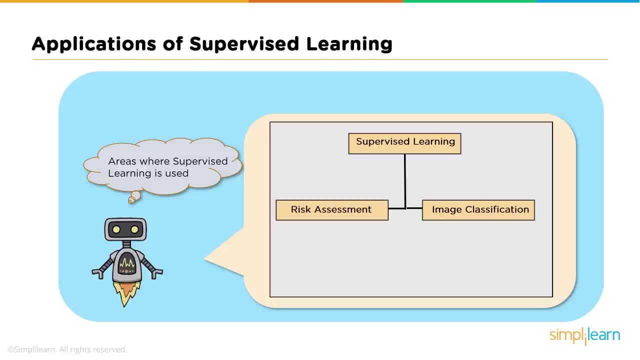 of tagged photos. So image classification is one of the key use cases of demonstrating supervised machine learning algorithms. Obviously, a lot more goes into all these, like convolutional neural networks, etc. Fraud detection, whether the transactions made by the user are authentic or not. 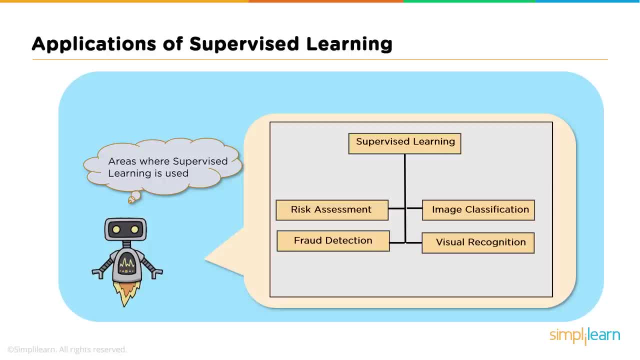 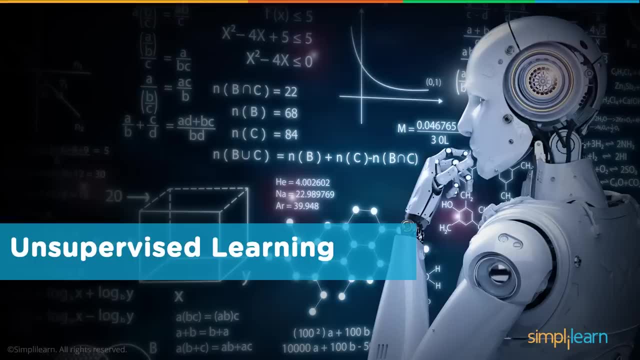 and visual recognition: The ability of a machine learning model to identify objects, places, people, and actions and images. Now let's quickly talk about unsupervised learning. In unsupervised learning, the machine learning model is to identify objects, places, people and actions in images. Now let's quickly talk about unsupervised learning. In unsupervised learning, the 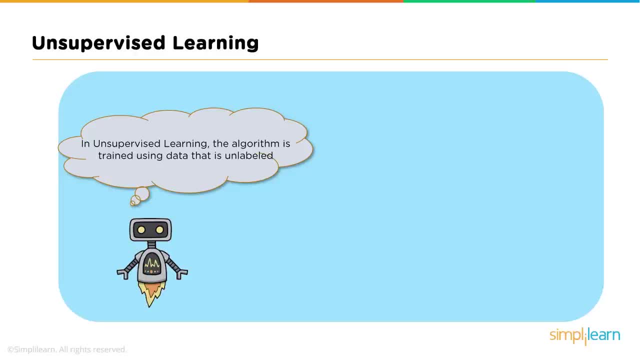 There is no supervision, that is, no training will be given to the machine allowing it to act on the data which is not labelled. Hence machine tries to identify patterns and gives the response. Let's take a similar example as before, but this time we do not tell the machine whether 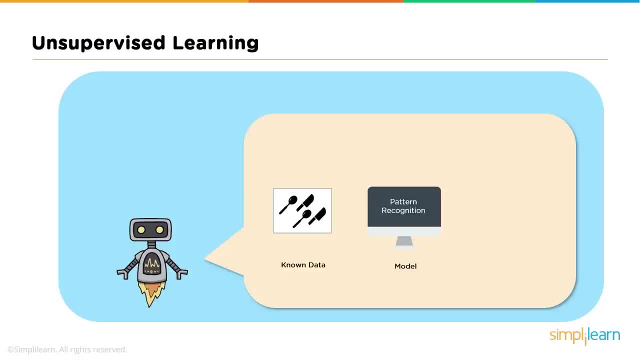 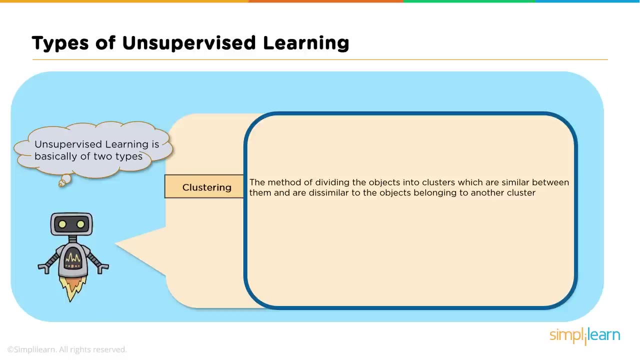 it's a spoon or a knife. The machine identifies patterns from the given set and groups them based on their patterns, similarities, etc. Again, unsupervised learning can be further grouped into clustering and association. Clustering is basically where the machine forms groups based on the behaviour of the 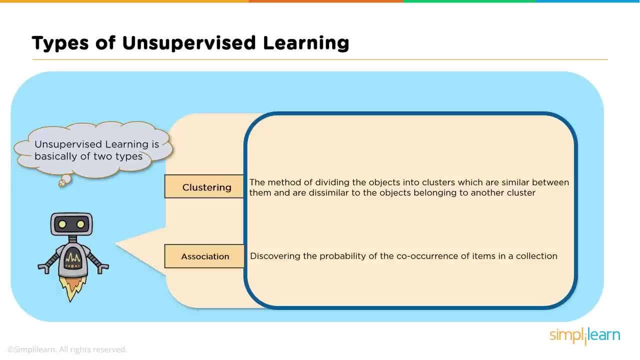 data. Secondly, association. It is a rule-based machine learning to discover interesting relation between variables in large datasets. For example, which customer made similar product purchases is clustering, whereas association is which products were purchased together. Now let's understand clustering further. Let's start with the help of an example. 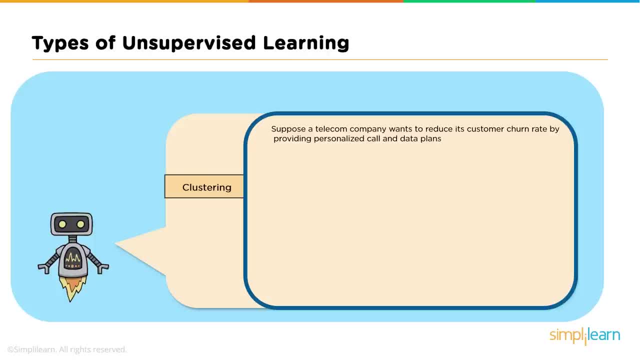 To reduce their churn rate. a telecom company studies the behaviour of the customers based on average call duration and internet usage and observes that while some customers call duration is quite high, others have heavy internet usage. The customers are grouped based on their observed behaviour and a strategy is adopted to minimise 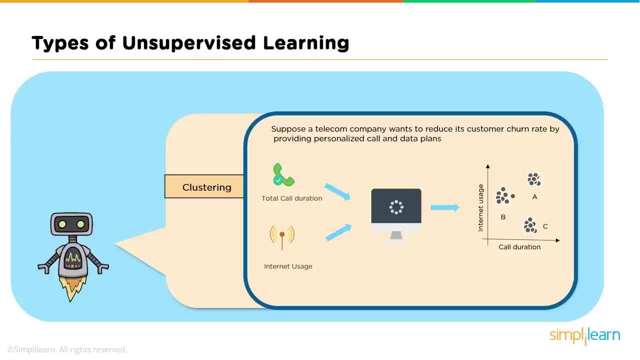 churn rate and maximise profit via suitable promotions and campaigns. As you can see in the chart on the right hand side, Clustering is a rule-based machine learning. Group A uses more data and also have high call duration. Group B customers are heavy internet users, while Group C customers have high call duration. 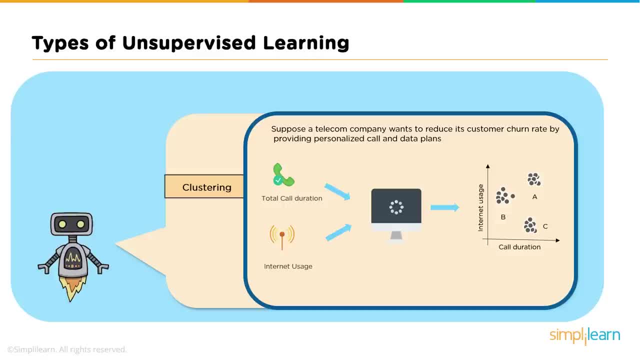 So Group B will be given more data benefit plans, while Group C will be given cheaper call rates to buy their loyalty. So this was the example of clustering. Now let's understand association with another example. Let's say customer 1 goes to a supermarket and buys these products, say bread, milk, fruits. 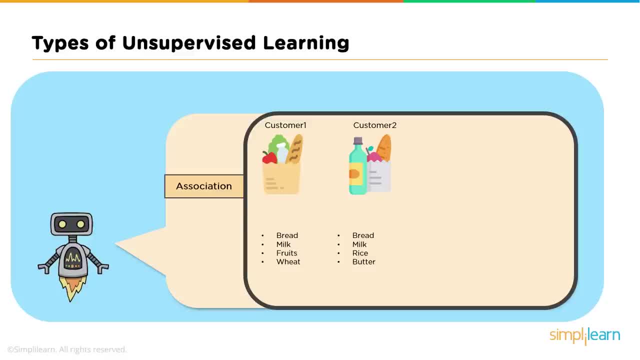 wheat. Then customer 2 goes and buys bread, milk, rice and butter. Now, when customer 3 goes and buys bread, it is highly likely that he will also buy milk. Hence relationship is established based on customer behaviour and recommendations are made. Now let's look at some real life applications of unsupervised learning. 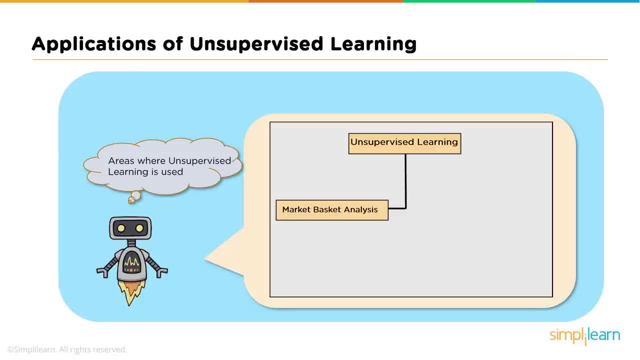 Market basket analysis is a machine learning model based on the algorithm that if you buy a certain group of items, you are less or more likely to buy another group of items. buy another group of items. semantic clustering: semantically, similar words share similar contexts. people post their queries on websites in their own ways. semantic clustering groups. all responses in: 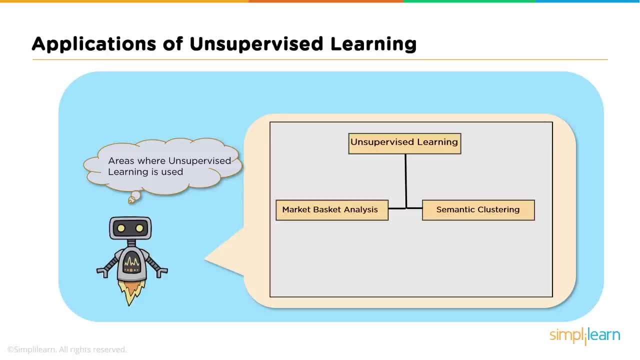 a cluster with same meaning to ensure that the customer finds the information they want quickly and easily. it plays an important role in information retrieval, good browsing experience and comprehension delivery. store optimization: machine learning models are used to predict the demand and keep up with the supply, also to open stores where demand is more and optimizing routes. 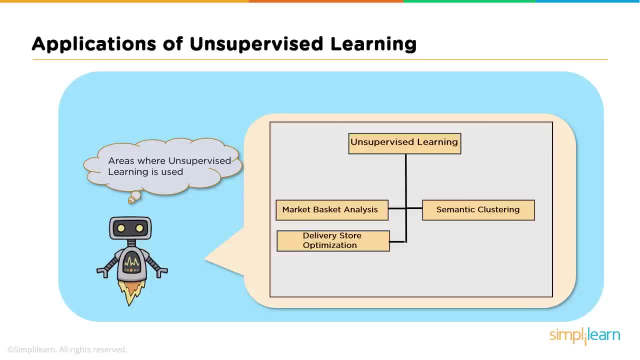 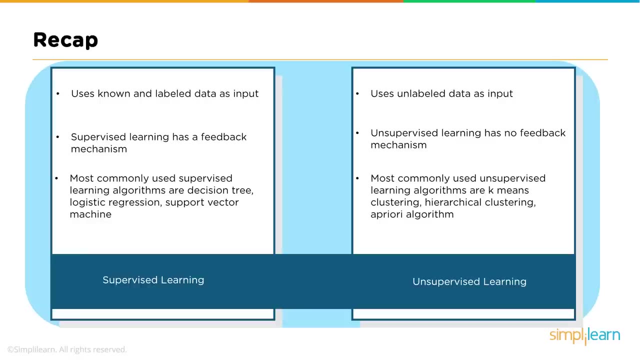 for more efficient deliveries according to past data and behavior. we can also use unsupervised machine learning models to identify accident prone areas based on the intensity of those accidents and the area in order to introduce safety measures. by now i hope you've understood supervised and unsupervised learning. for a quick recap, let's see a few differences between the two. the most